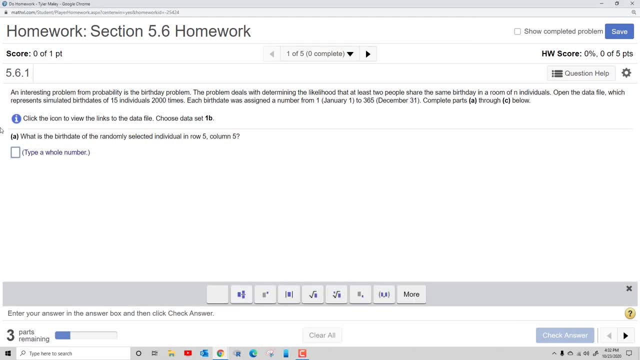 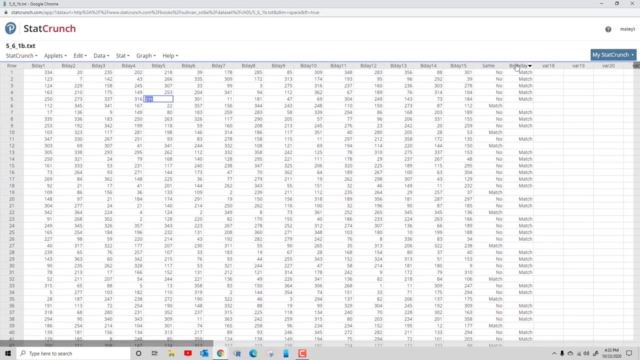 Alright. so it says: did the first simulation result? at least two people share the same birth date. So if we go back to the, the dataset notice this same birthday is like split into columns, but it still works. so if it says no and then match, that means in other words, if there's a no in this column is, even if it's personalities, yes, and that makes sense. That makes sense. So if we go back to the, the dataset, and scroll the way to the data1 file- a data set like split intoomed of 2, then there's single Pi has the same pairs. So that means that number 10,став doesn't match to 1, there's 2column has the same up compared, which has a different sum. If people enter the same number and people do the same number, This data gate kind of gives you a data case. So moving on, 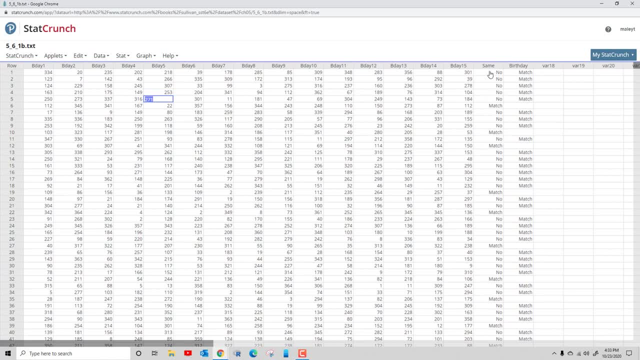 In other words, if there's a no in this column, it means there were not two birthdays the same out of 15 people, And if it says match, then that means that there is right. So looking at the first simulation, the first row, there's no match, right. 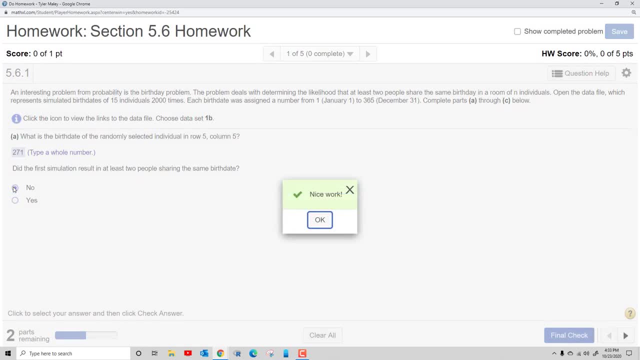 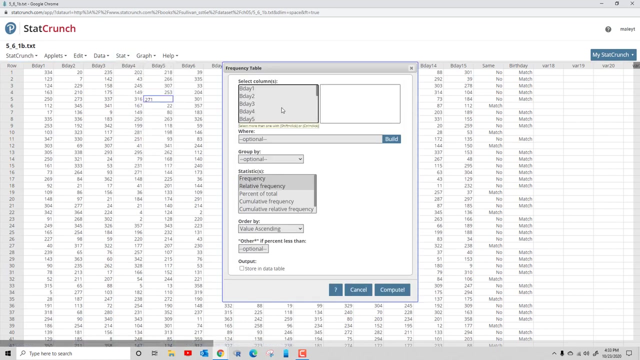 So we would say no. And then part B says: based on the simulation, what's the probability that at least two people share the same birth date? right, So to do this we can get a frequency table. So we go to stat tables frequency and we want to do that for the same column. 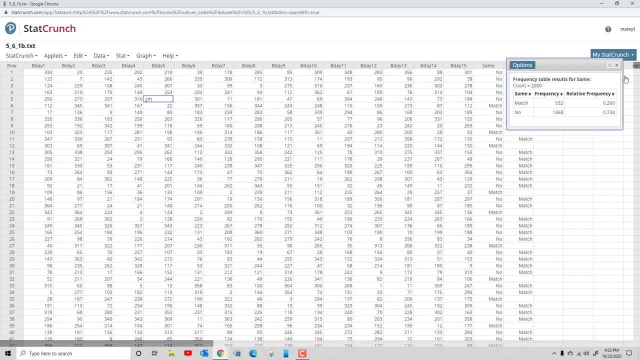 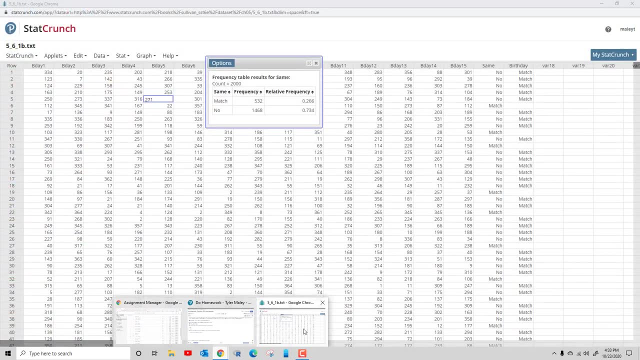 And I'm going to leave it with frequency and relative frequency hit compute. So then, the idea is: so we were looking at the probability that they do have the same birth date. right Yeah, that they will share the same birth date. 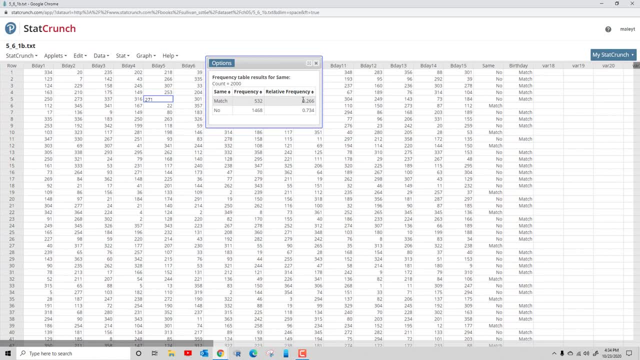 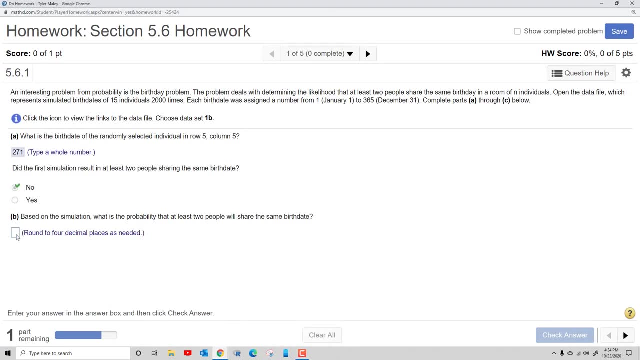 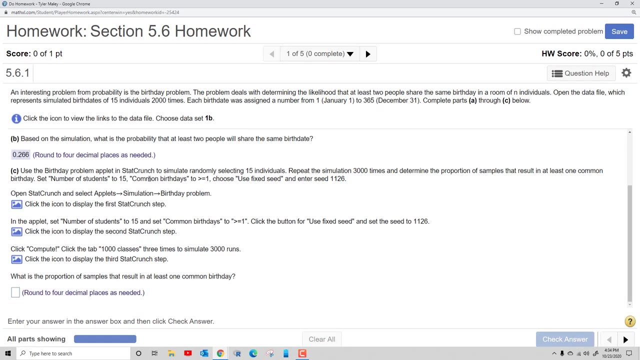 So we would want the match column right, So that relative frequency would be the probability right, So 0.266.. All right. So then now we're doing another simulation. It tells you step by step and you can click on these pictures for screenshots to help you, if you know, if you need that. 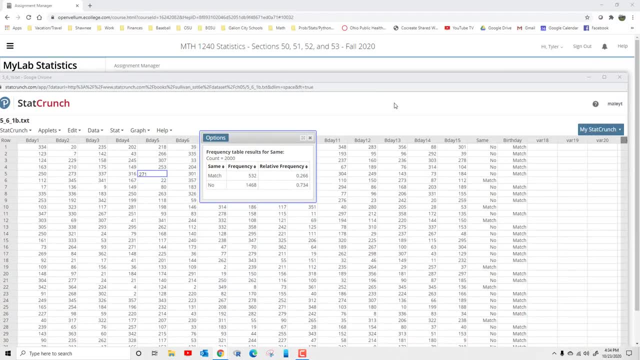 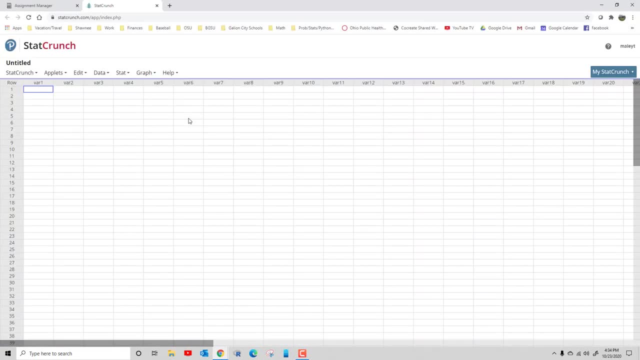 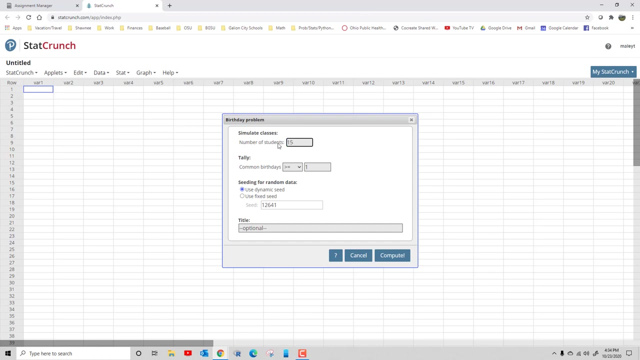 So I'm going to go over here. I'm just going to make a new Data table. So the directions say to go to applets and then simulation and then birthday problem, And then it tells me to put 50 in for the number of students and to leave the common birthdays to greater than or equal to one. 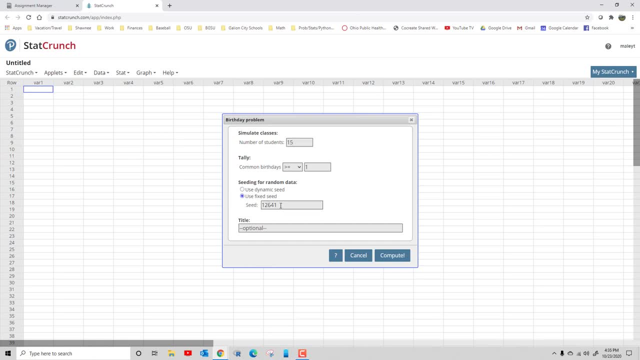 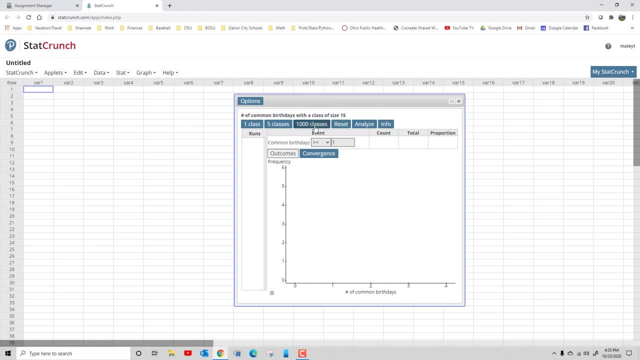 And then we're using a fixed seed of 1126, right, So I need to fill that in. It tells me to hit compute, And then it tells me to put 50 in for the number of students, And then it tells me to hit 1,000 classes three times, so that way we're doing 3,000 runs, right. 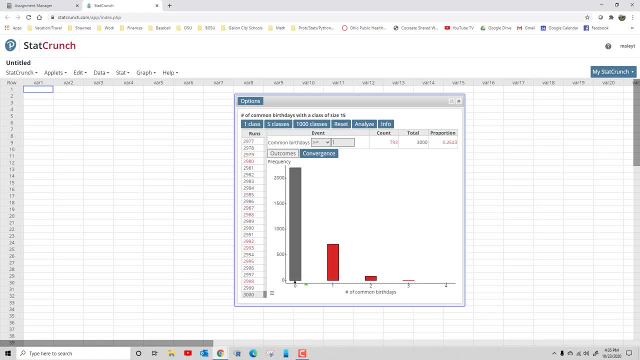 So I hit that once, twice, three times, And then the answer I'm looking for is: what is the proportion of samples that result in at least one common birthday, right? So that would be this value here in the table, this proportion. 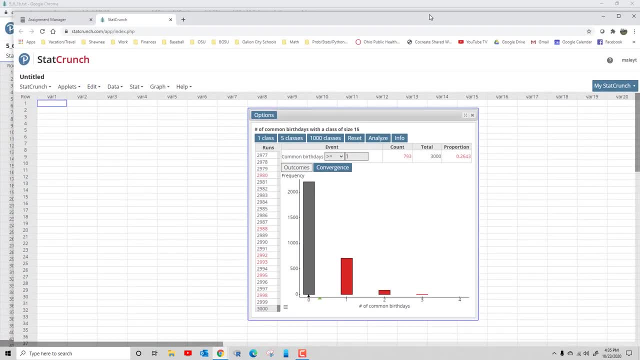 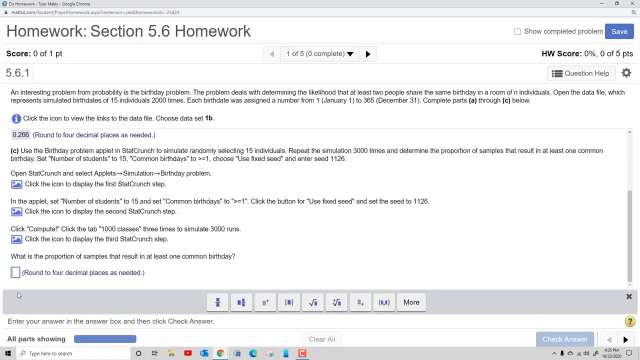 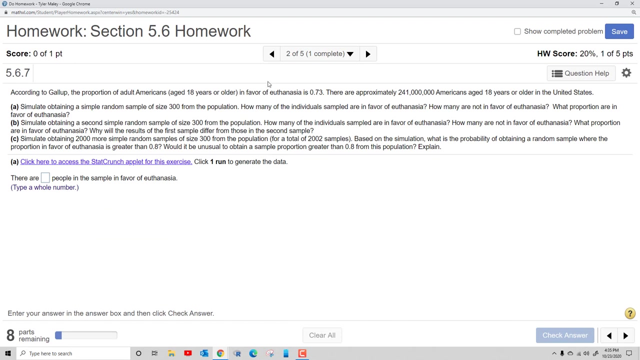 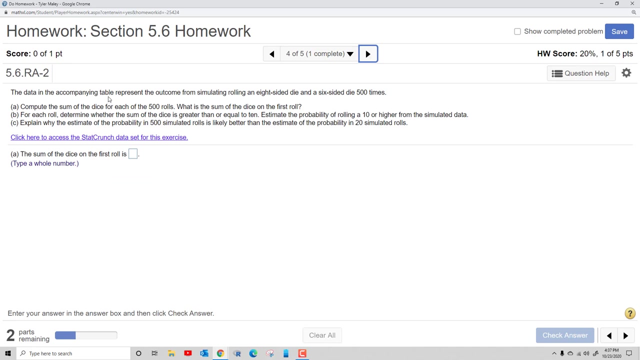 So I just need to type that in. All right, 0.2643 is what I had, and I got it right. Now I'm moving on to the next question, right, All right? so the next problem that I wanted to do is question four. 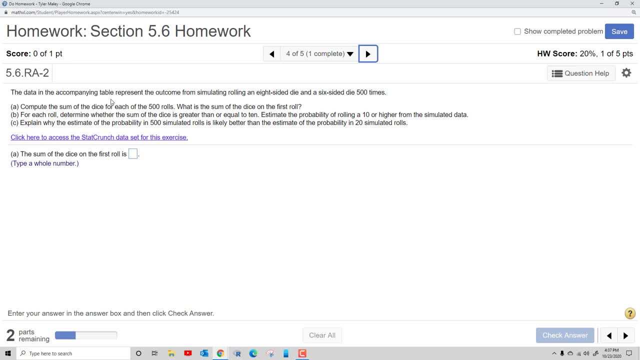 It says. the data in the accompanying table represent the outcome from simulating rolling an eight-sided die and a six-sided die 500 times. Part A is to compute the sum of the dice for each of the 500 rules. What's the sum of the first rule? 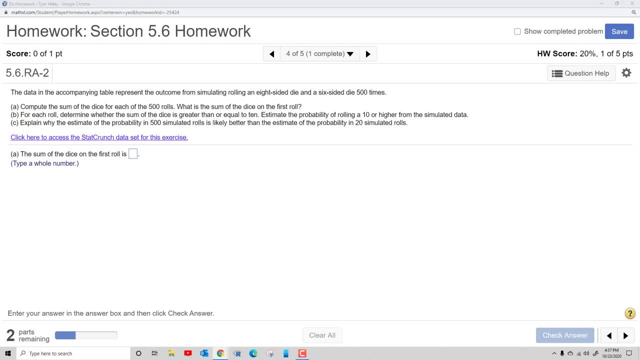 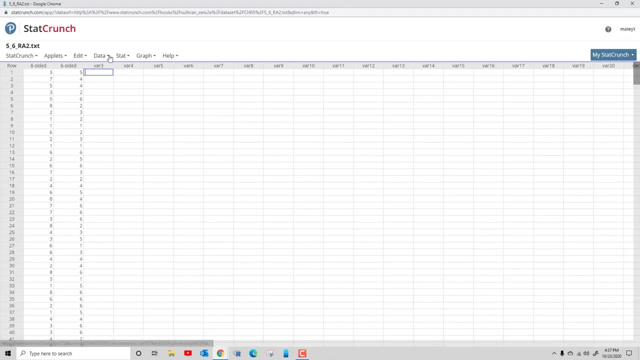 So if you click on this link it'll pull up the data table And then we want to input a new variable here where it's calculating the sum. So if I go to Data Compute and then Expression and then you click Build, 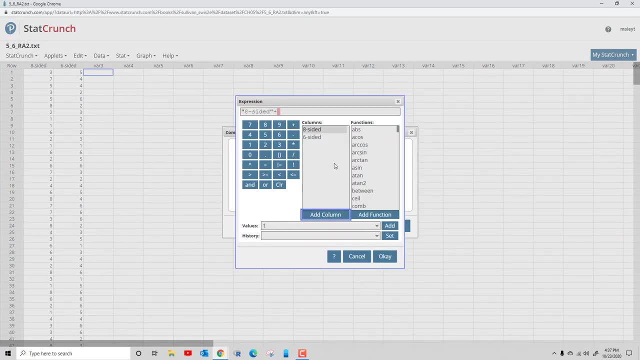 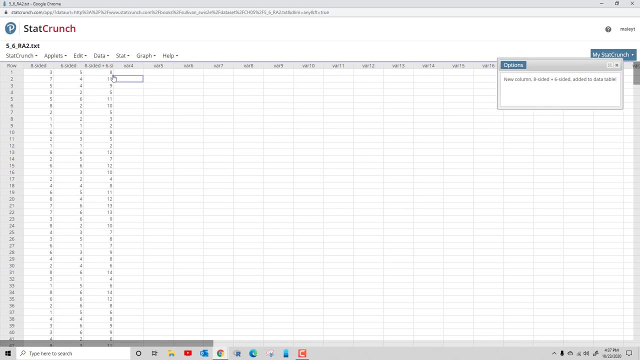 then what I want to do is take the eight-sided column and hit Plus, and then the six-sided column and hit Add Column and then hit OK, hit Compute And then. so what's happened here is we have each of these numbers now. are the sum of the two dice right? 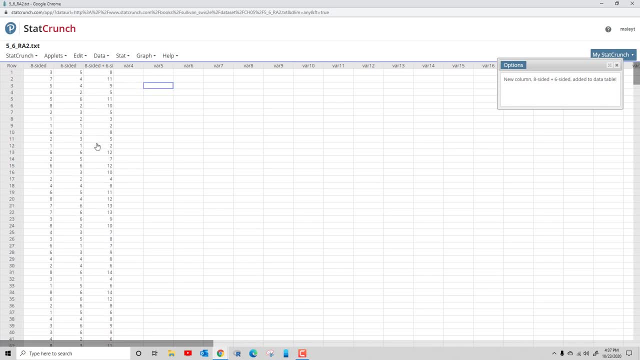 So, like this number is 5 plus 4, which is 9.. It did that all the way down for me, right? So what I'm looking to do is it's asked: you know what's the sum on the first rule, right? 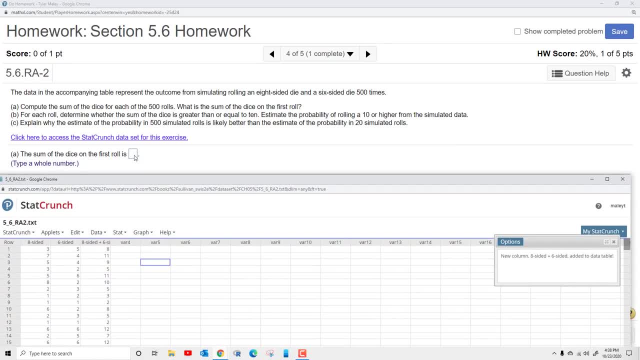 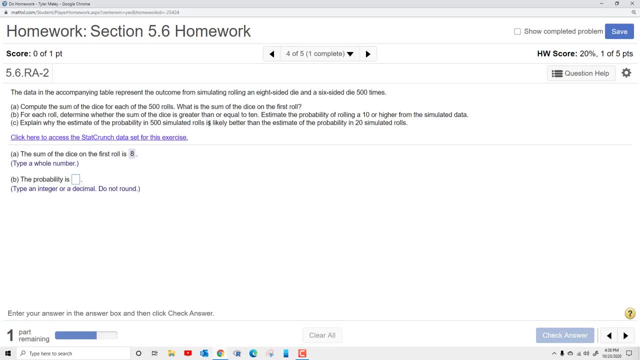 So the first rule is 3 plus 5, which is 8, right, So I would click this here: 8.. Part B says for each rule: determine whether the sum of the dice is greater than or equal to 10.. 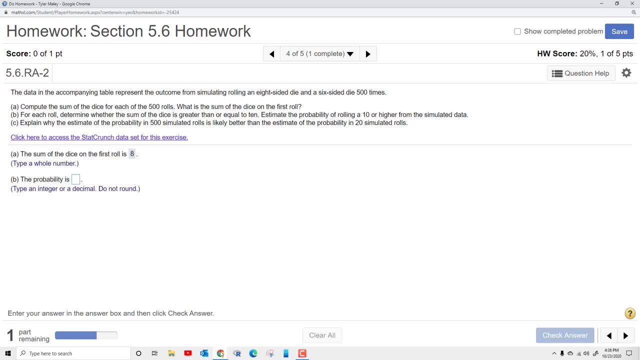 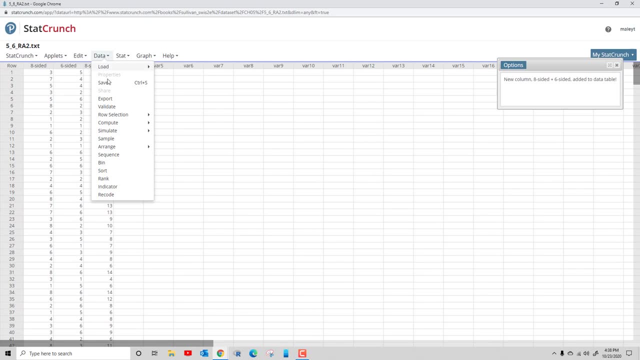 Estimate the probability of rolling an eight-sided die. All right, So if I'm rolling a 10 or higher from the simulated data, right? So something I can do here is I can go to Data and then go to Ben and then I'm going to click Use Cut Points and we want to use 10 as my cutoff point. 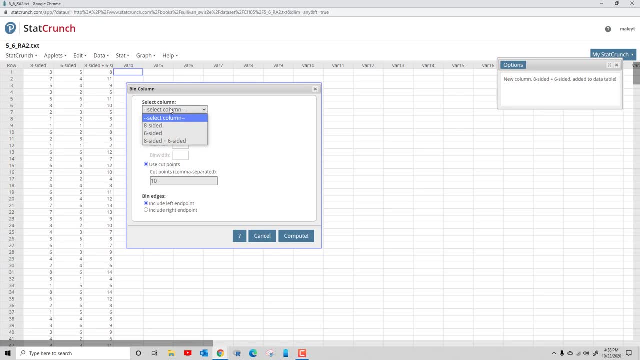 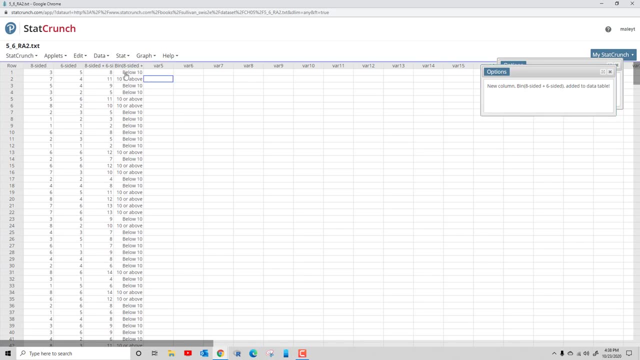 And if I hit Compute- oops, I got to click the column, So we wanted the eight-sided plus the six-sided- Hit Compute and then. so now what it's done is: it's identified if the sum is below 10 or 10 or 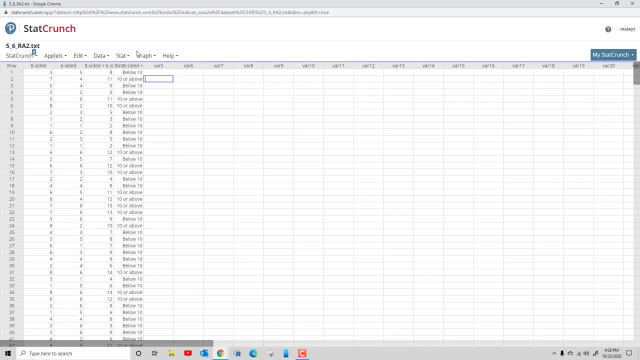 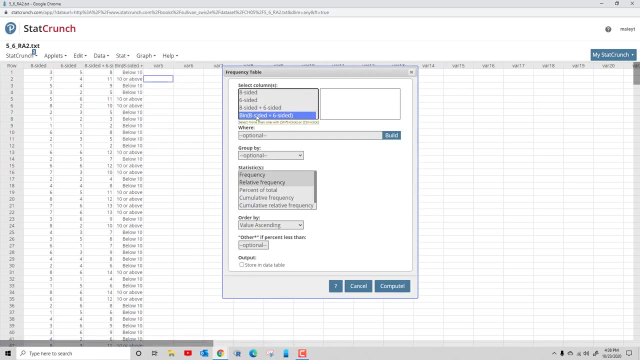 or above. all right, So we're looking for the probability of 10 or above. So if I go to Stat Stat Now and then Tables and then Frequency, I want to do this, Ben, eight-sided plus six-sided variable Hit Compute. 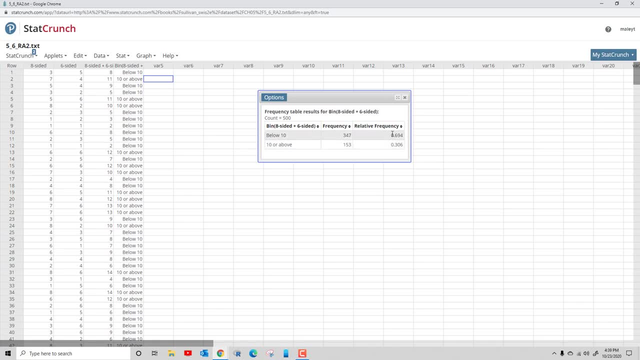 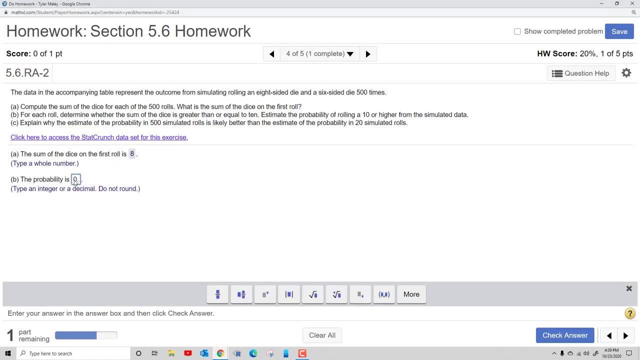 So then the probability of 10 or above would be this relative frequency .306.. I think it was 306, right? Yep, All right. So then you know. it says why is the estimate using 500 simulated rules likely better right. 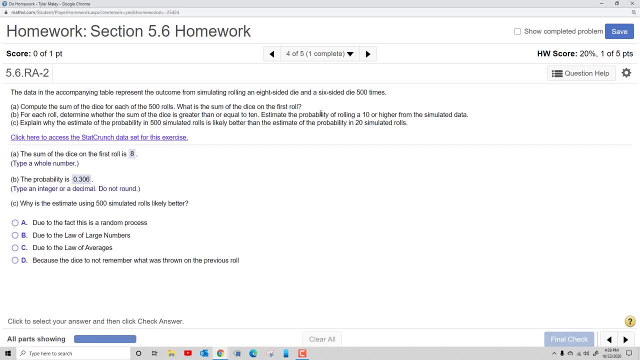 So why would using 500 rules be better than using 20 rules, right? Well, that's because of the law of large numbers, right? Hopefully you don't forget that law, right? The idea is, the more trials we do, the closer it's going to get to the true theoretical probability, right? 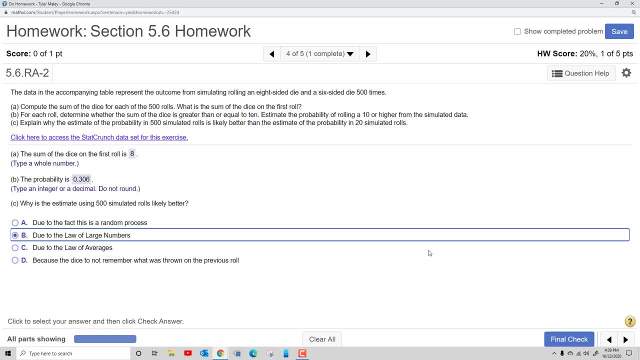 So we want to do it. We want the end value to be large, right? So doing it 500 times is much better than just doing it 20 times, right? And actually in the previous question I didn't do this. You can do it.